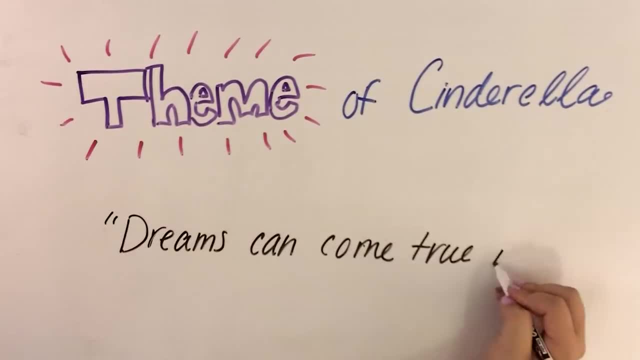 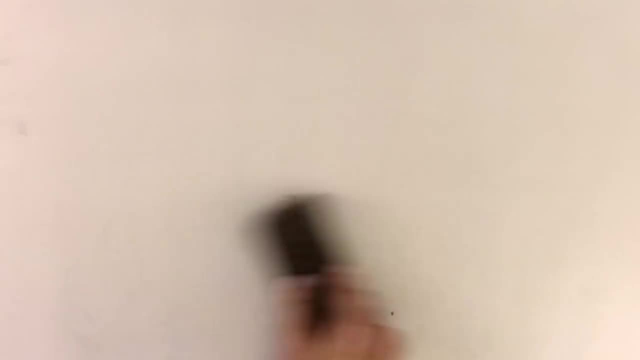 chosen theme for Cinderella is: dreams can come true if you don't give up. So we need to find literary elements that prove that this is a meaning in the story. Let's start with plot. In the movie, Cinderella eventually gets her dream of going to the ball because she didn't 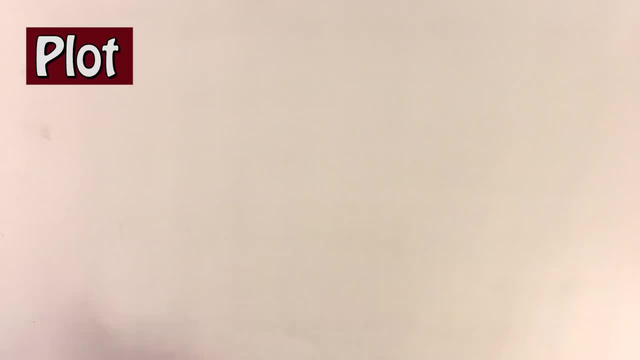 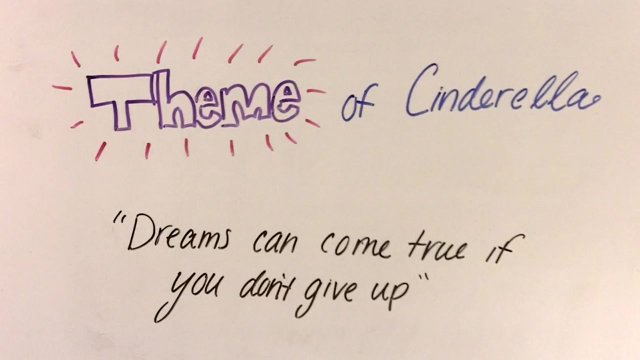 give up, despite the obstacles that her family caused. Prince Charming also gets his dream of finding Cinderella after traveling his whole kingdom with a glass slipper. Both of these examples are events in the plot that support our bigger meaning. dreams can come true if you don't give up. But you don't want to stop with only one literary element. 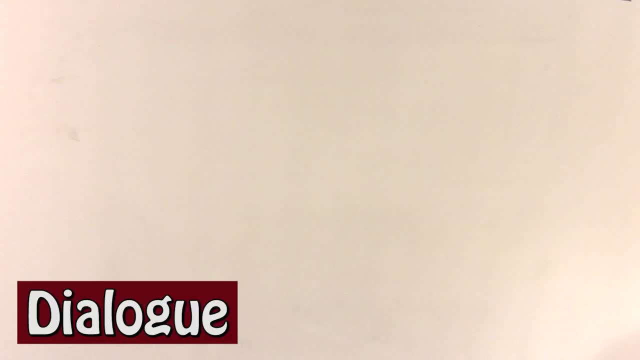 Try to push it further. Another element we could use is dialogue. We could discuss the words in the song, the language, the text, the words that are said in the song, the. a dream is a wish that your heart makes, which is from the movie. 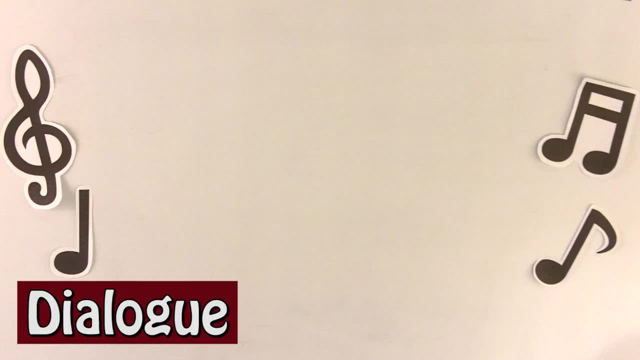 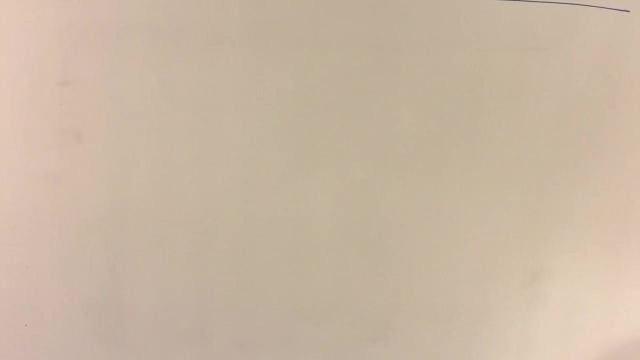 we'd be able to pull out specific lines like: No matter how your heart is grieving, if you keep on believing, the dream that you wish will come true. This is another piece of our analysis. We could also use the literary elements- symbolism- to prove our theme by talking about how the glass slipper symbolizes a 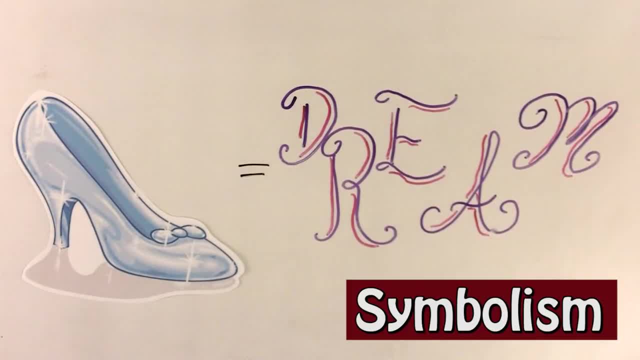 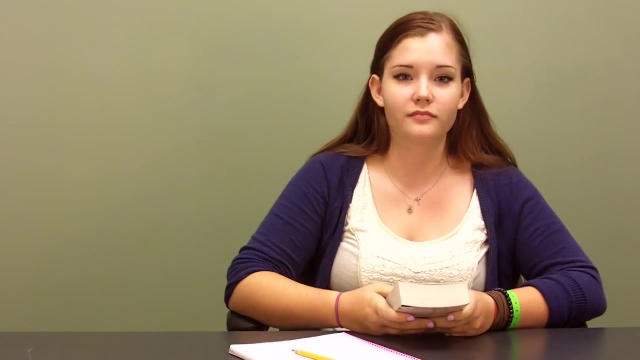 dream that has come true. After all, shoes made out of glass are certainly more dreamlike than realistic, but somehow they become true enough for Cinderella to wear them to the ball. As you can see, we're studying all of these literary elements to think critically about the whole story. That's literary analysis. You. would use the word dream to describe a dream. but you would also use the word dream to describe a dream. As you can see, we're studying all of these literary elements to think critically about the whole story. That's literary analysis. You would use 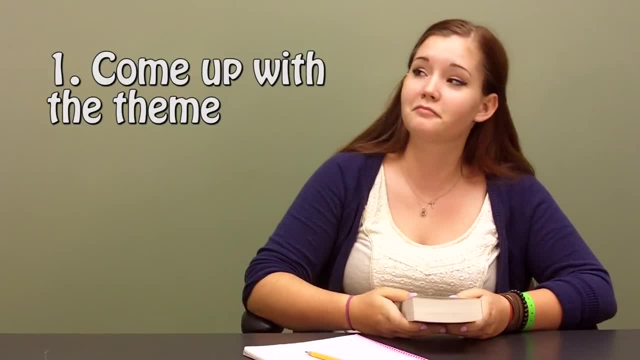 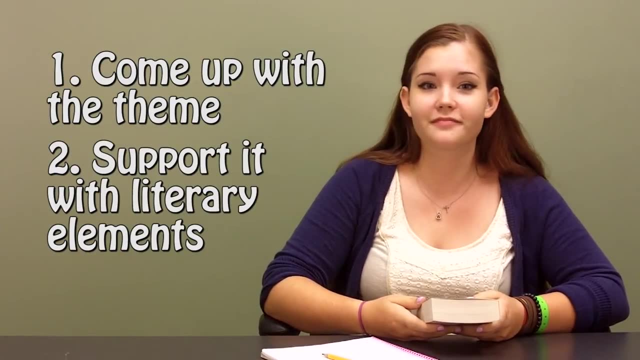 this same process to analyze any text. First come up with the theme, which again is a bigger meaning of the story. Then pick out literary elements that prove that your theme is true. Want to learn more tips for succeeding in college? Stop. 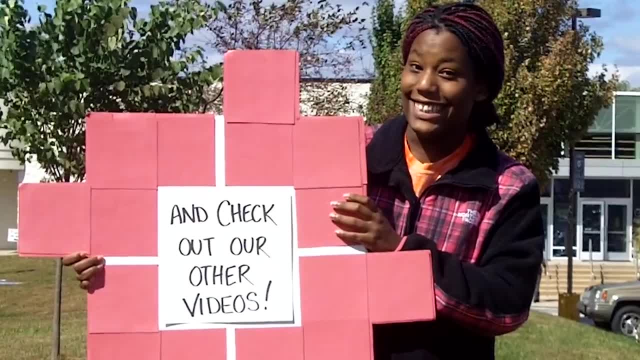 by the Learning Center at your HACC campus to talk with a tutor. And don't forget to check out our other cool online videos. See you next time.